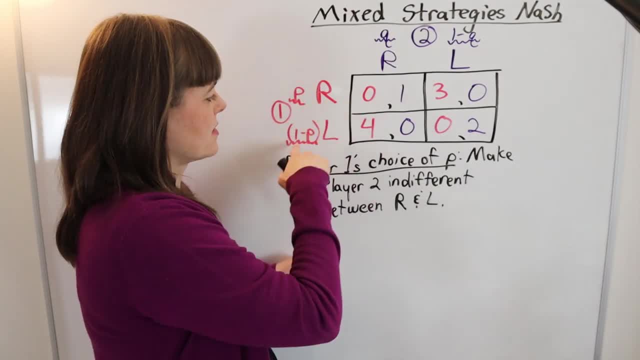 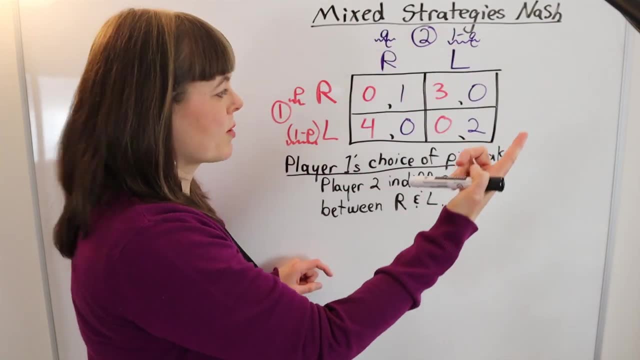 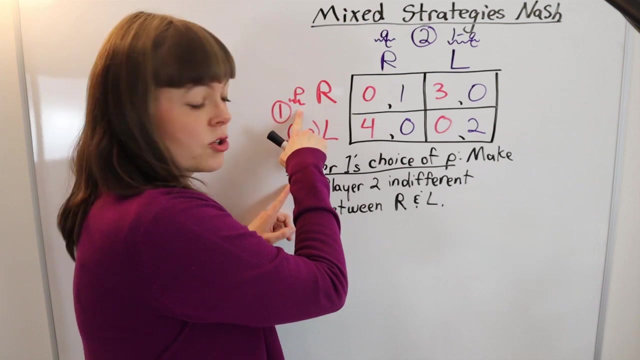 Player one goes right with probability P and left with probability one minus P. Player two goes right with probability Q, left with probability one minus Q And, of course, the rule that you use to solve these problems is that player one chooses P, the probability of going right. 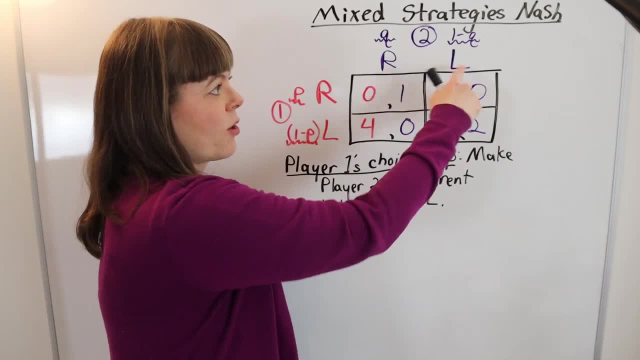 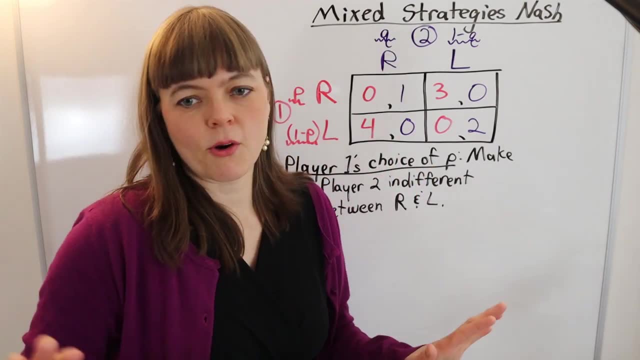 in order to make player two indifferent between going right and left. Now that is a little bit counterintuitive. but once again, in this video, I'm just showing you the math, I'm not showing you the intuition. So let's set this up. 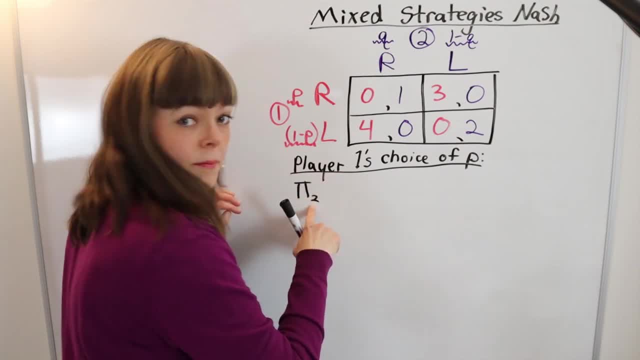 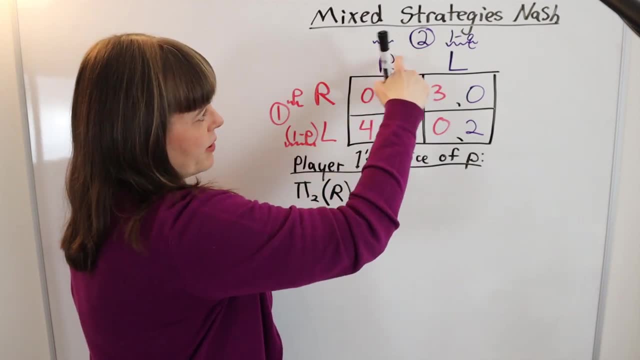 So we'll do the payoff to player two of going right. That's going to be our first player two, So we'll do the payoff to player two of going right. That's the first equation we set up, And if player two goes right, 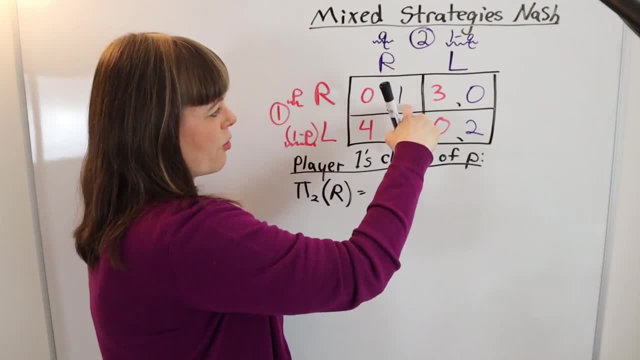 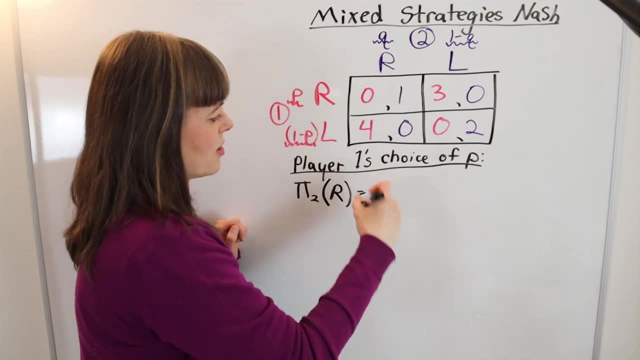 well, player two is either going to get one or zero And, of course, what's the chance that player two will get one? That's chance P, the probability that player one goes right. So we've got probability that player one goes right. 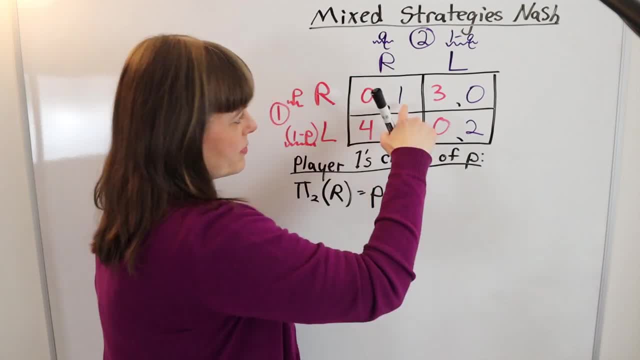 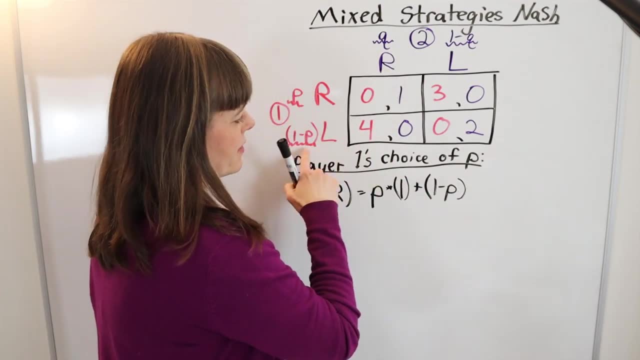 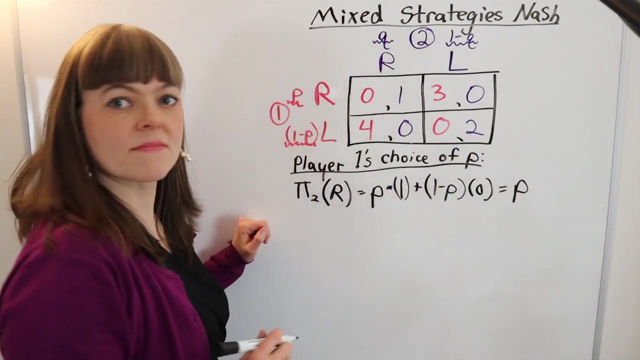 times the payoff to player two if player one goes right, plus the probability that player one will go left. one minus P times the payoff to player two, which is zero. So this simply equals P. And now that we've got the payoff to player two of going right, 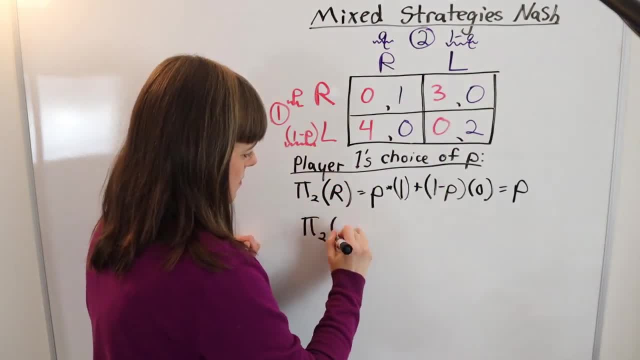 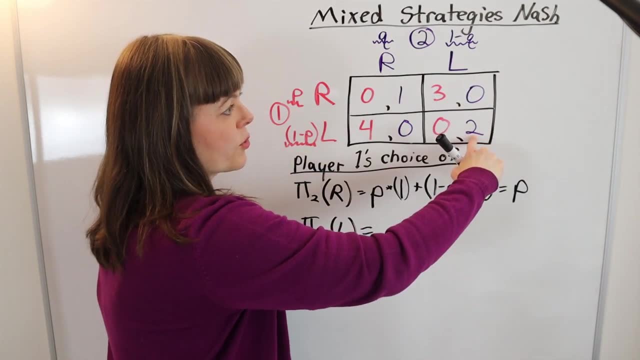 we're going to set up the payoff to player two of going left, And that is going to be equal to well if player two goes left, we know that player two will either get the zero or the two, And the probability of getting each is given by 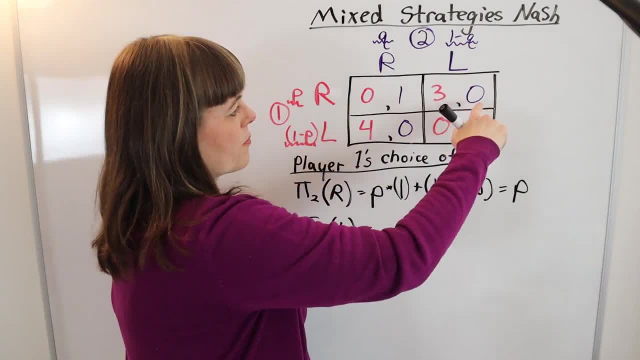 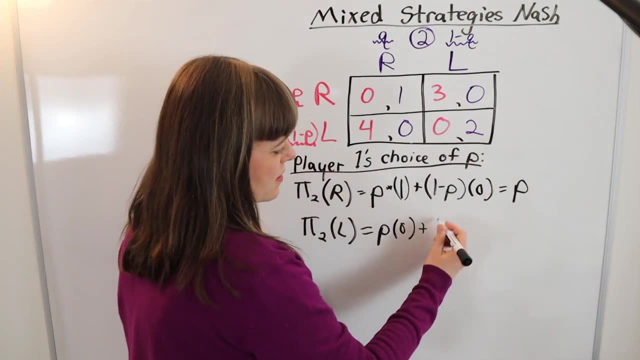 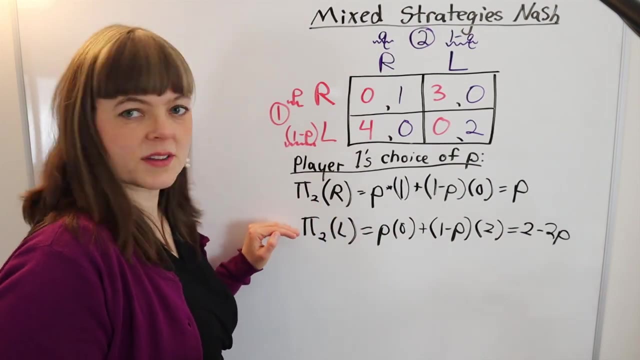 the probabilities over here of player one choosing that. So probability of this times payoff if we end up up here, plus probability of getting this times the payoff if we get this And of course, when. is player two indifferent between going right and going left?